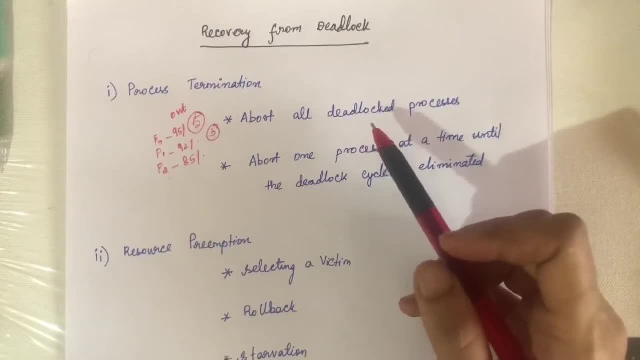 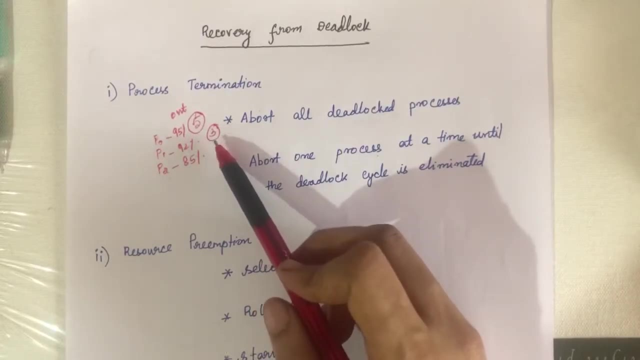 the process termination. So we need to detect what are all the processes which are suffering deadlock. after directing it, we need to kill all the processes. for example, if you are having five processes out of which three processes are suffering from deadlock, like p0, p1 and p2, you are suffering from deadlock but p0 has. 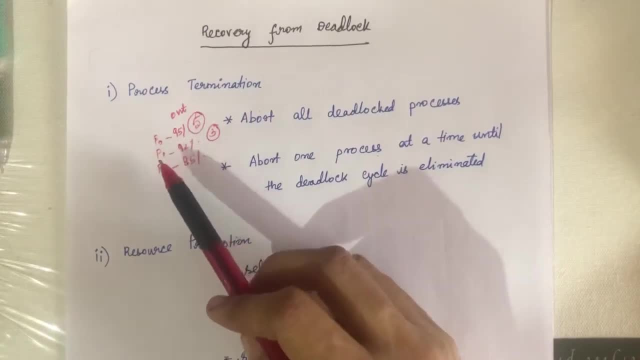 already completed 95 percentage of its execution, p1 already completed 92 percentage and p2 already completed 85 percentage. but in this time, if we have directed the deadlock, we need to kill all these processes: p0, p1 and p2. okay, so because of this, resources are wasted, like CPU memory time. everything is. 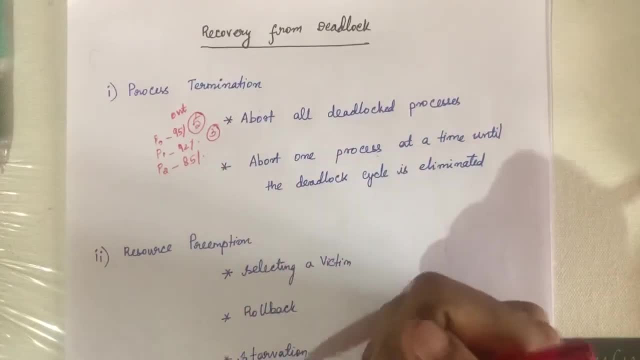 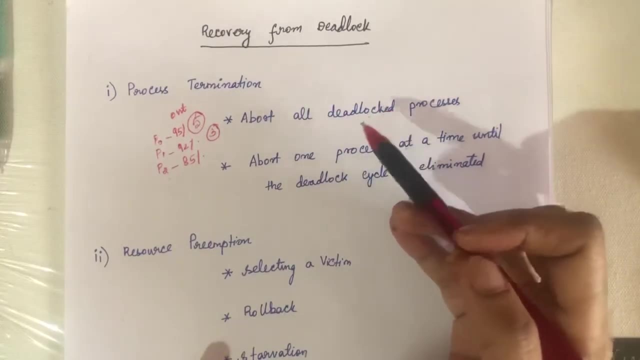 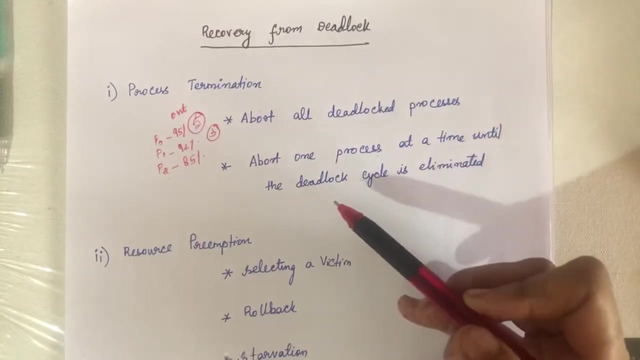 wasted and again, after killing this, again we have to start from the scratch. so this type of aborting all, deadlock the process is costly one. the second one is abort one process at a time until the deadlock cycle is eliminated. so in this way, what we have done is that in this way, we have selected all processes out of. 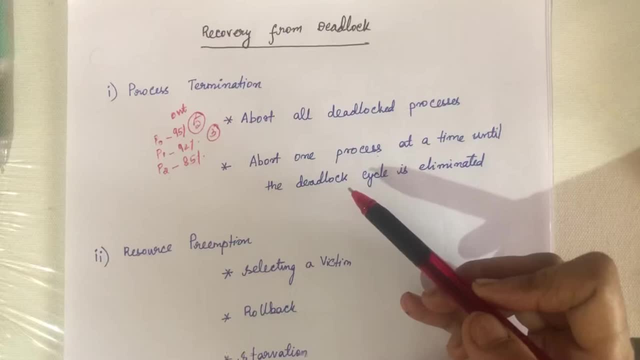 going to do is we need? we will be killing one process again. we will be using deadlock detection algorithm and we will check whether deadlock cycle occurs or not. if deadlock cycle occurs, then we will kill another one process again. we will use deadlock detection algorithm to check whether you have the cycle or not. this process is being repeated because of repeatedly checking. 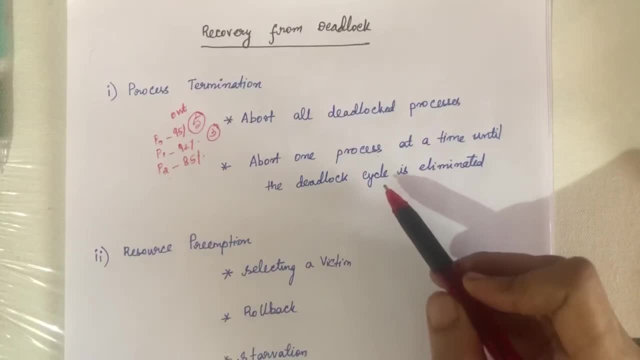 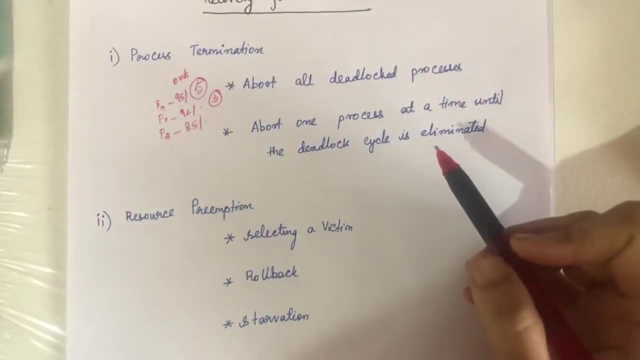 deadlock detection algorithm. overhead incurred in this way is very high. so these are all the disadvantages of using these two ways. if we want to reduce the cost incurred in killing the process, what we can do is that we can check the priority of a process, so whether it is a low priority. 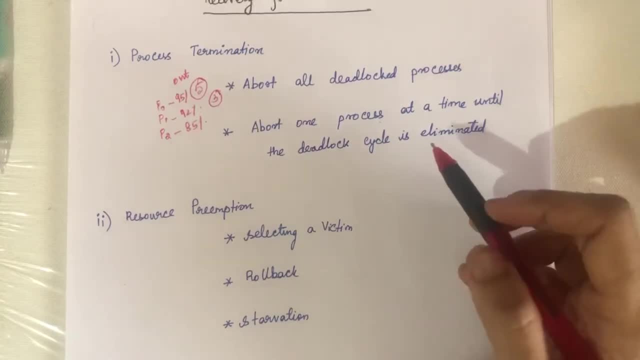 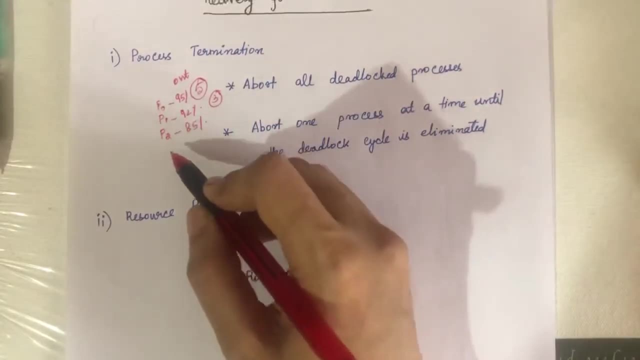 process or high priority process. so we can, based on that, we can kill the process. the second is, we can calculate how long the process is completed. for example, if you are having p4 processes, which p3 process, which is having just completed only 10%, among all this thing, we can kill the process which is having the low, which which is having 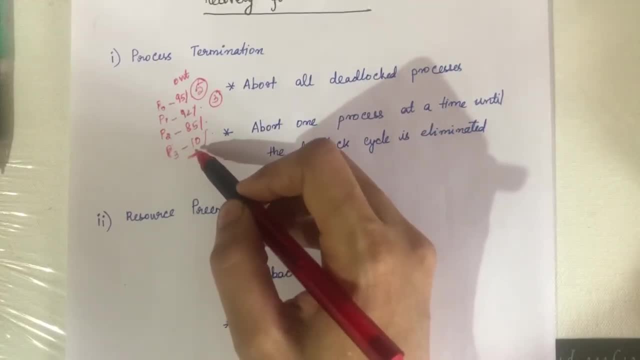 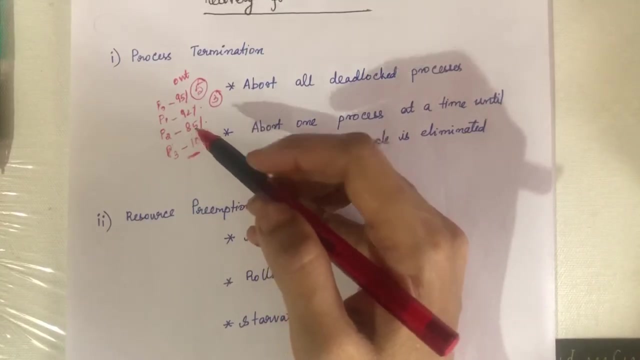 this low percentage. that means it has it. it has completed only 10 percentage of its execution, so we can kill p3 instead of killing p0, p1 and p2. so like this we can do it and we can also check the factors like whether it is an interactive or whether it is a batch process. based on this,